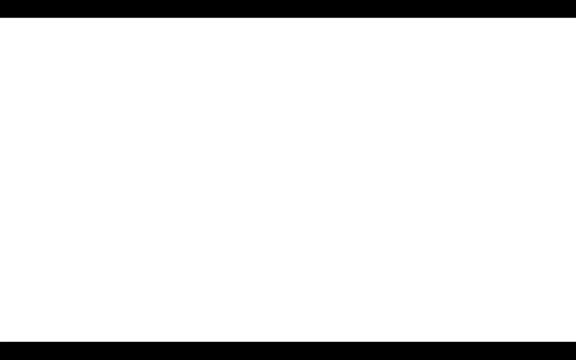 this will be slight repetition, but let's get started. So let's say we have an abstract program which prints the word hello and the first module, which means your program, is known as tokenizer, right Or lexical analysis. Sometimes this module is called lexer or scanner. and what's the purpose of the tokenizer? 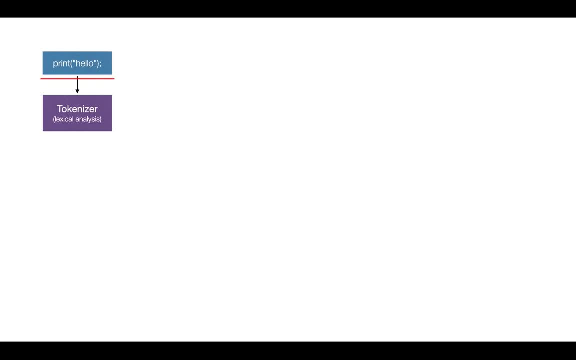 As we can see here we have characters p, r, i and t. This means that we have theiot in the corpus of the variables, open parentheses, etc. and it's not very convenient to work with individual characters. So the purpose of the tokenizer is exactly to group this set of characters and to produce the 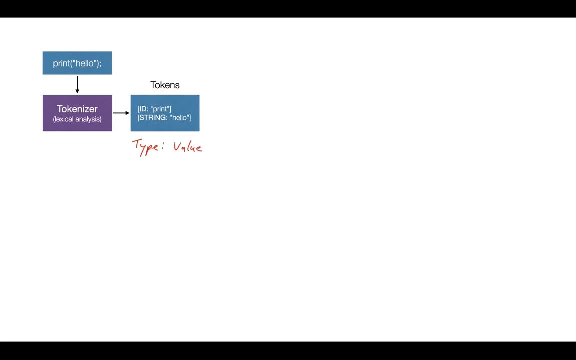 first intermediate representation, known as stream of tokens And, as you can see, token has type and a value and this value is also called a lexeme. So in this case we have two tokens: the identifier with the value print and the string token with the value hello. 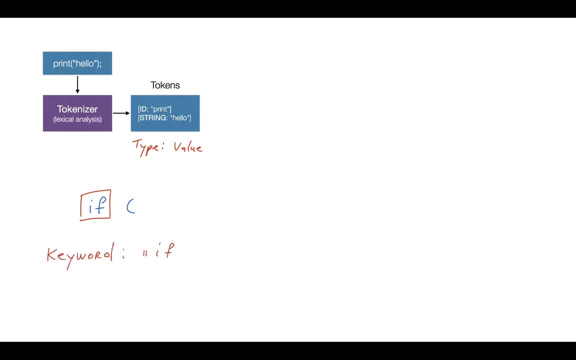 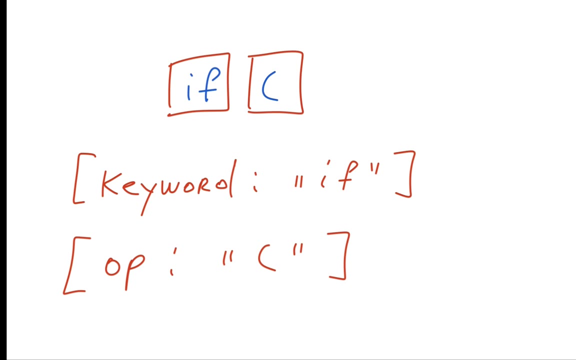 that Tokenizer doesn't validate whether our program is syntactically valid. right, it might be completely syntactically invalid, As in this case we have the program, which consists of two tokens, the keyword if and the open parenthesis, and for us, for readers of this code, it's obvious. 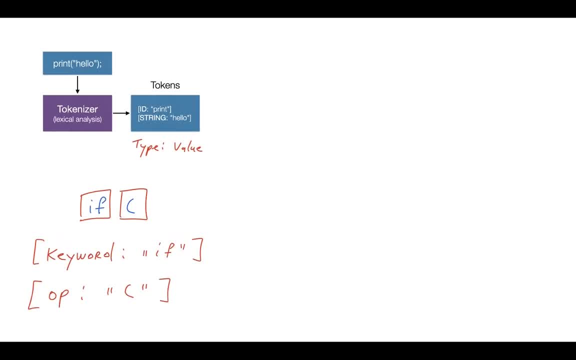 that this code is invalid, But Tokenizer will normally be able to obtain two tokens again: the keyword if and open parenthesis. Now the module which actually validates whether our program is valid- syntactically valid- is known as parser, and this is exactly the purpose of. 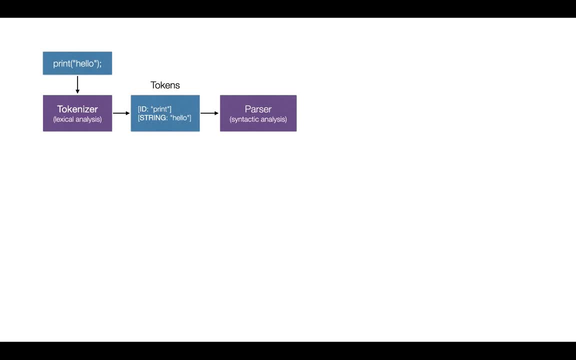 our class, We'll be focusing specifically on this module and we'll implement and talk about all the different algorithms used for parsing. And in theory, the purpose of the parser is specifically the validation, that is, whether the string is accepted by your grammar or not. but in practice, 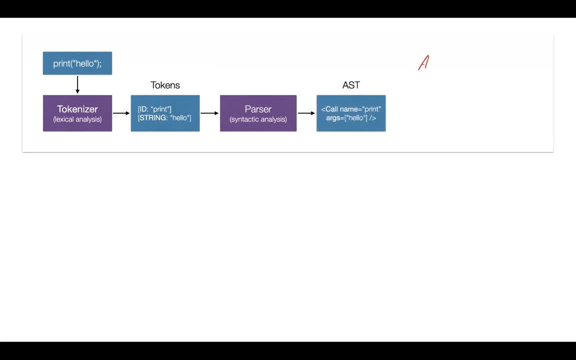 parser produces the next intermediate representation is known as abstract syntax tree right, or AST for short. Now, this is a tree representation of our program and this is something what we can already feed to an interpreter or to virtual machine and to obtain the result. And again in this class we will build a parser which consumes some program in string. 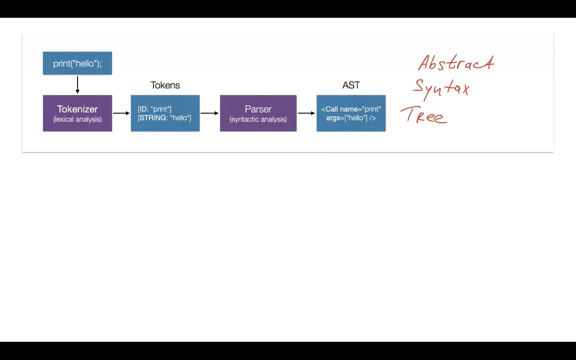 representation and produces specifically the AST. Okay, so let's take one more example of the AST: x equals 10 times 5 and plus y. So a possible AST for this program might be an assignment operator which has left-hand side and right-hand side, right, and on the left-hand side we see the identifier x. 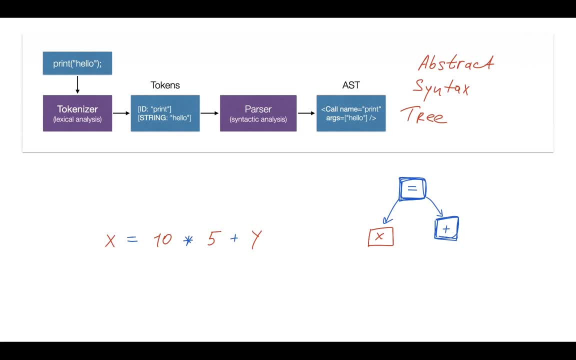 and the right-hand side. here is a complex expression itself right, this is a addition which has left-hand side, which is multiplication, again with the left-hand side 10 and right-hand side 5, the right-hand side for the addition, that is the identifier y. Okay, so that is the example of the AST. 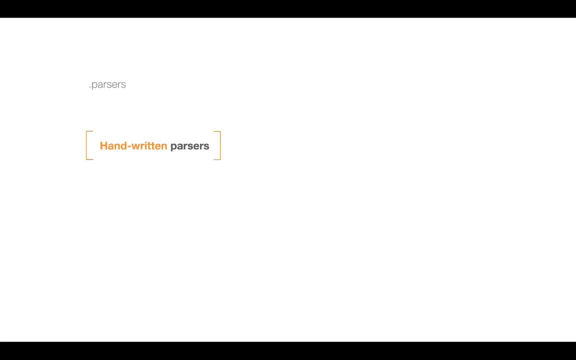 And when we talk about parsers, we differentiate the handwritten parsers and automatically generated parsers. Now, for the handwritten parsers, we mainly have the implementation, which is known as recursive descent, and there are multiple implementations with backtracking, with predictive. most of them are recursive. that's why it's called recursive descent. 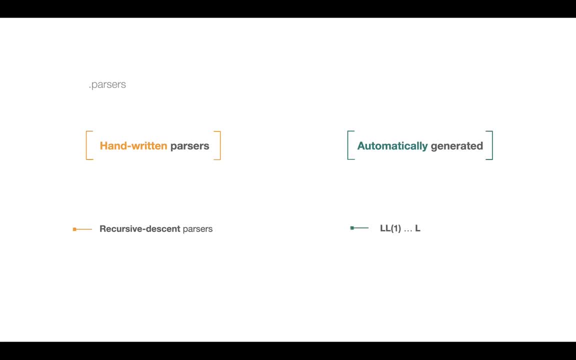 recursive descent. But in general the parsing process can be automated right And there are tools which are called parser generators which can take a grammar of your language and produce a fast, non-recursive, that is, table-driven parsers which can scan in linear time And as an example you can take a look at. 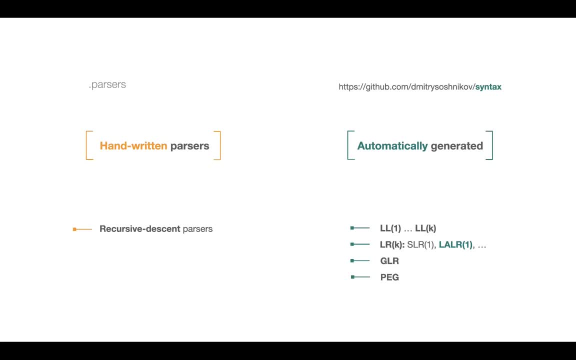 this tool called Syntax, which is language-agnostic parser generator. What is language-agnostic? It means you can write a grammar once and then produce multiple targets for different languages. for example, JavaScript, Python, Rust, there's Python, integration, Ruby and many others, And we'll be actively. 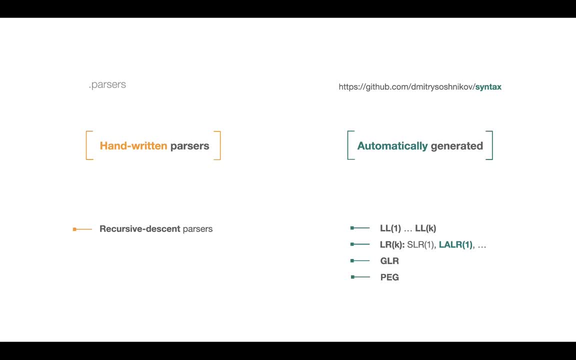 using Syntax tool in this class to build our parser. Okay, so the parsing process relates to text processing. right Text consists of sentences. sentences consist of words or tokens, lexems, and so this is the exactly what we start with, and we'll talk about symbols, alphabets and languages. 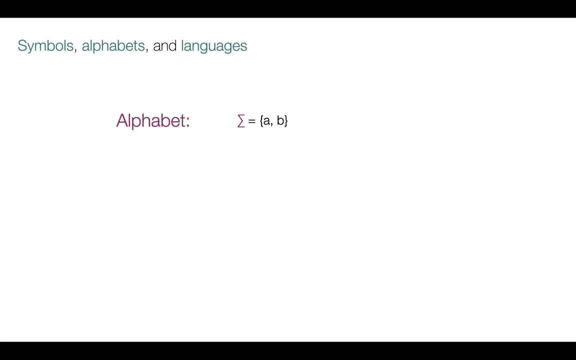 Now, first of all, let's talk about alphabets. Usually, in parsing process, the alphabet is denoted with the Greek letter Sigma, And let's say we have this alphabet consisting of only two characters, A and B. right, An English alphabet consists of 26 characters. Russian alphabet consists of 33. 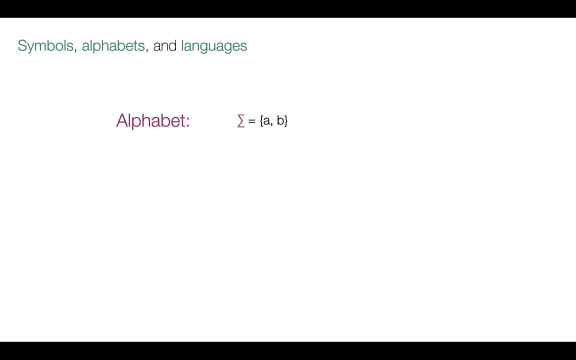 characters. in this case we have only two. So we say that the alphabet is a set of characters And a language is also a set, but in this case it's a set of letters, a set of strings consisting of the characters from the alphabet. For example, 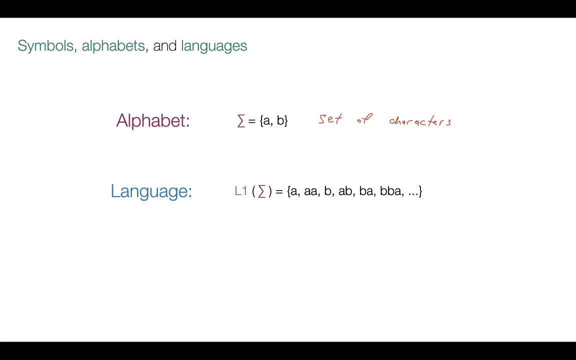 the language L1 here consists of any possible strings of any length, of any permutations from the symbols, from this alphabet And, as you can see, we call such languages as infinite, since we can generate again all possible permutations. However, we can continue adding some restrictions, for example of: 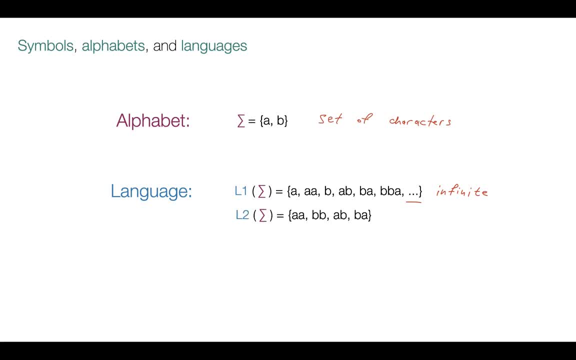 the language L2,, specifically that all the strings in this language should exactly have the length 2.. And in this case the set of strings is actually finite. Now the main takeaway here: once we start applying restrictions on the language, we form exactly the grammar right. The grammar is a set of 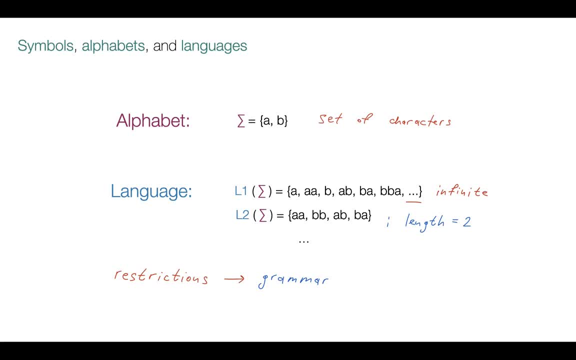 restrictions on top of the alphabet for the specific language. So let's take a look. what is the formal grammar? Again, all the languages have grammars. right, There is English grammar, there is again Russian grammar, and programming languages have grammars. Technically, a grammar is a tuple of. 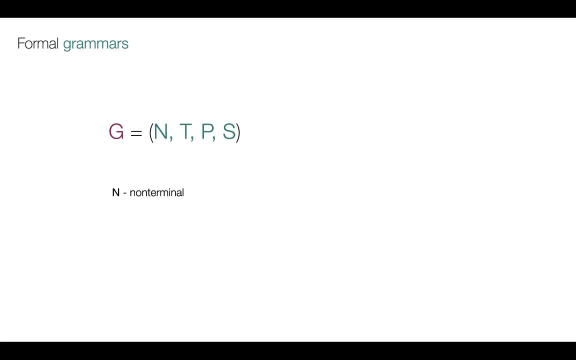 four elements: N, T, P, S. Let's take a look what it is On the right-hand side- here we see an example grammar, and let's take a look what specifically each component means here. So the N, which stands for non-terminals, or the 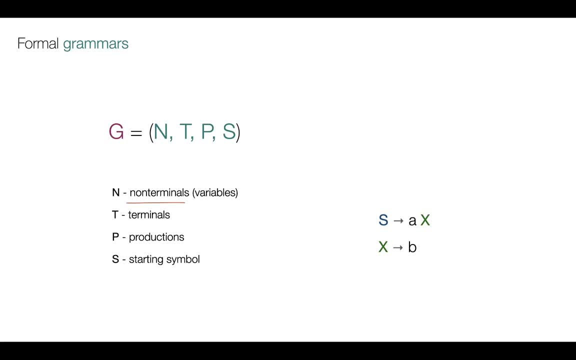 variables defines a set of symbols in our grammar which can hold some value right, Which can hold either a single letter, a single character or a subset of other characters. And in this case we have two variables: the variable S, which is the starting symbol in this grammar, and the 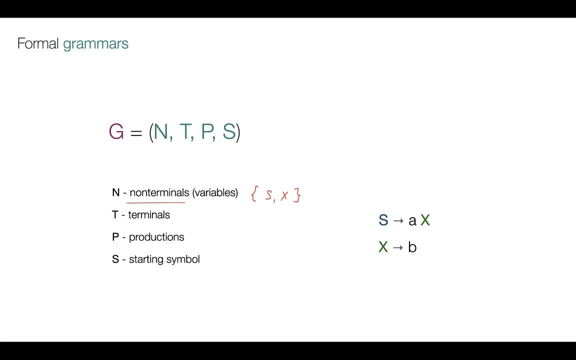 variable X which, as you can see, can be rewritten with the value B, So once again, a variable can be replaced with the value it holds. Now, in contrast, the terminals are the actual symbols which appear in our strings, in our programs, as is right. It's not a special variable, but exactly the specific character, That's. 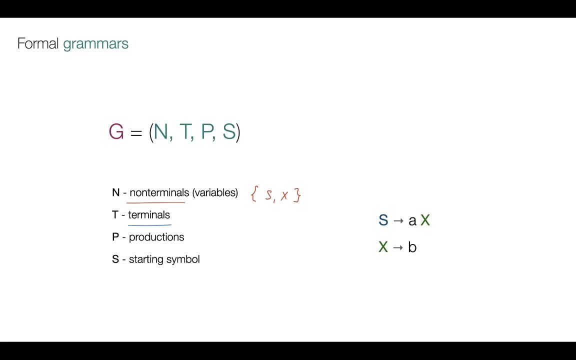 why it's called terminal. that is final symbol, And in this case we have two terminals again and a subset of other characters. And in this case we have two terminals again and a subset of other characters. And in this case we have two: the character A and the character B. Now the P component defines the set of 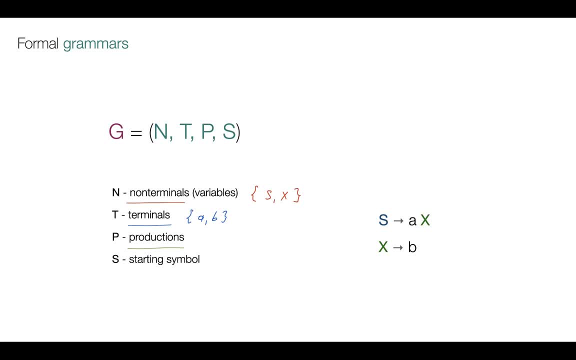 productions or the rules. in this grammar These are exactly restrictions or rules which form our language right, Which specifically tells how the language is structured. And final component in the grammar is the starting symbol. This is just the first production, the first symbol we start our analysis from and 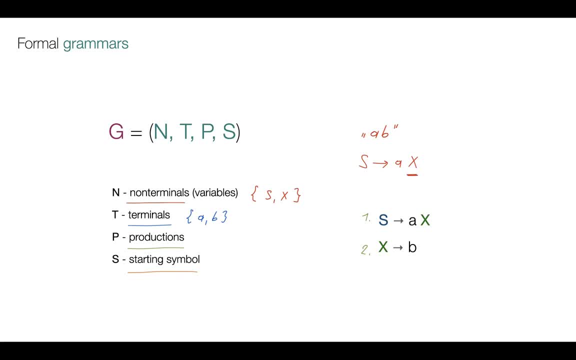 start our derivation process, that is, the replacing some variables followed by the values they hold. So, once again, this is the grammar and this tuple, and TPS is enough to describe any complex programming language: context-free, context-sensitive, regular, as we will see shortly. And let's move further. And when? 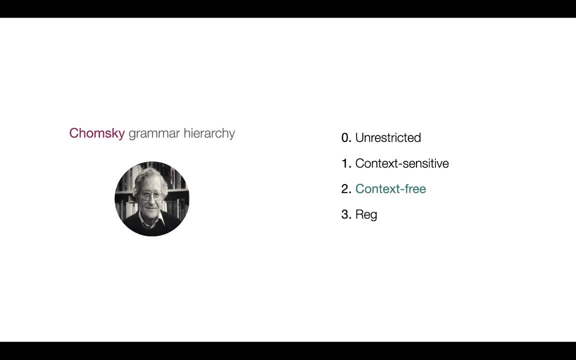 we talk about grammars, there is so-called Chomsky grammar hierarchy, right defined by the Noam Chomsky and who made a great contribution to the formal grammars, to programming languages and natural languages processing, And Chomsky defines this hierarchy consisting of four types of grammars: The unrestricted. 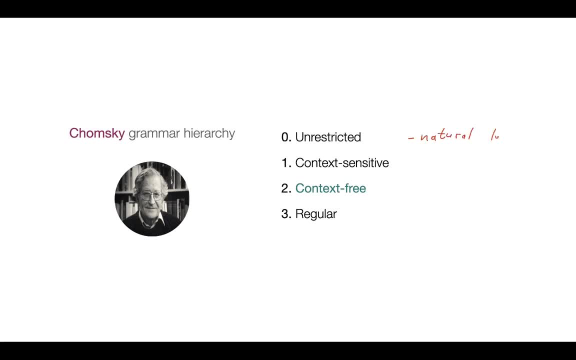 grammars, that is, type 0, are used mainly for natural languages processing. The context-sensitive and mainly context-free are used specifically for parsing programming languages And the regular grammars are used for parsing regular expressions. To reiterate, in this class we'll be focusing specifically on 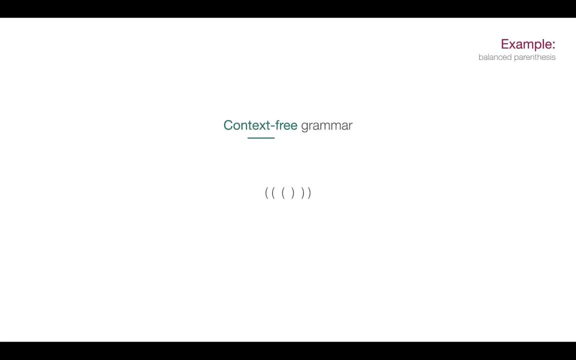 the context-free grammars. So what is context-free grammar? Why context-free grammar? Well, it turns out the regular expressions which we studied in the automata class are not enough to parse a programming language. The simplest example- right balanced parentheses- is not possible to parse. 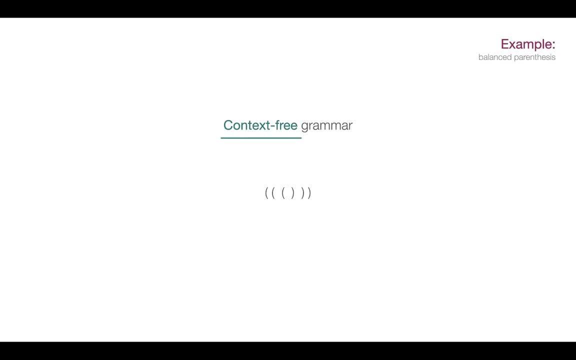 with classic regular expressions based on the finite automata. Now, on the other hand, the context-free grammar, which is abbreviated as CFG, is trivial here. Let's take a look. So, first of all, we replace the inner S by itself. that is, again parentheses S, parentheses again. replace S by itself. 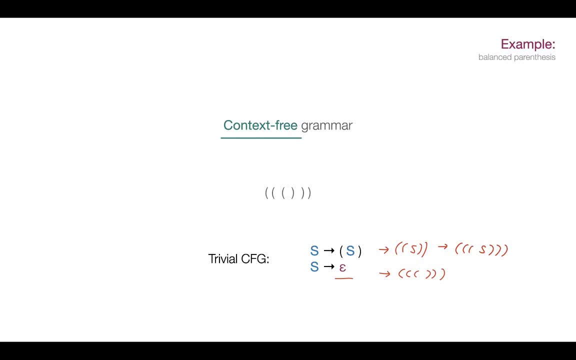 Finally, we eliminate the S by the second rule, the symbol called epsilon, and literally it means we can eliminate the symbol altogether. So again, this is a trivial, context-free grammar, while it's not possible in regular grammars. And now let's give a formal definition of what a context-free grammar is. Now, first of all,